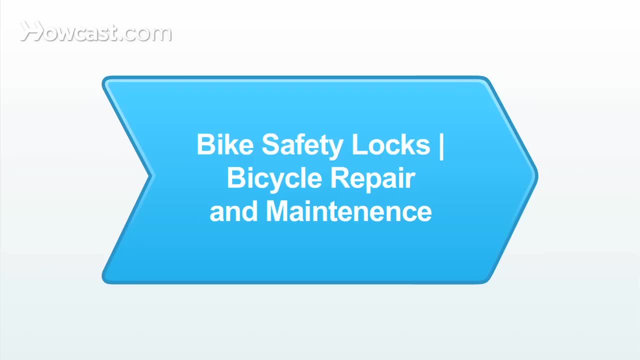 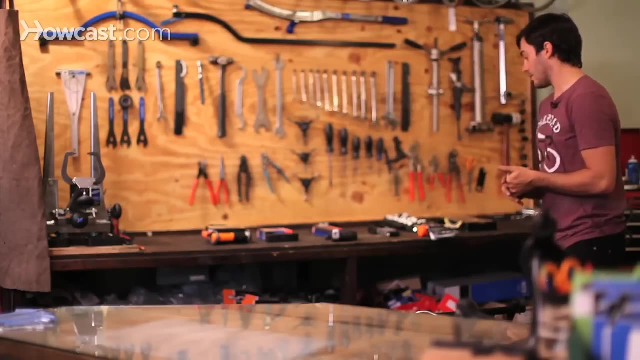 Okay, so now we're going to talk about locking up your bicycle in New York City. This is definitely one of the highest cities for theft for bicycles, especially So you want to make sure that you secure your bike because you don't want to come out and have your wheels missing or your frame missing or your entire bike missing, because that is never fun. So let's go through the different locks. So in New York City, you want to make sure that you're getting a lock. that's usually around $60 or more. 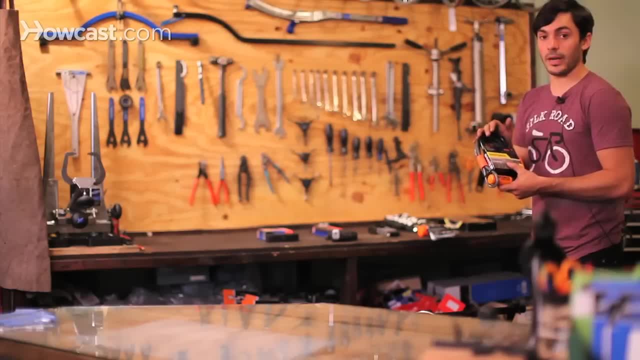 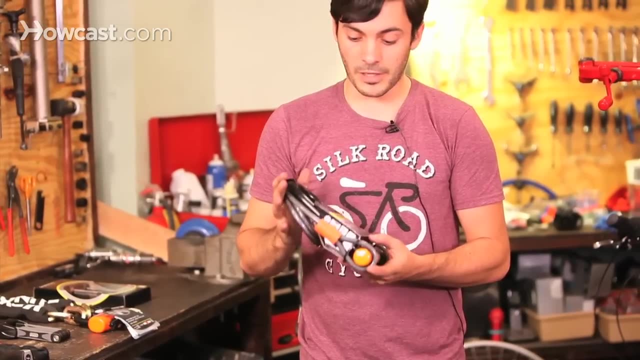 And basically what that's going to assure is that you have the proper security rating. So all the locks are made out of different materials. If you get a lock that's too cheap, it's going to be really easy to break Here at the shop. with the tools that we have, some of these locks can break really really. 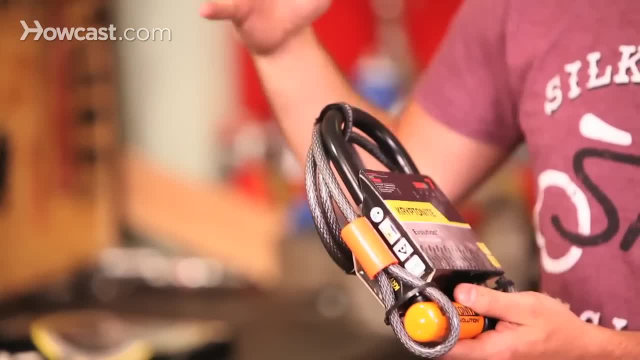 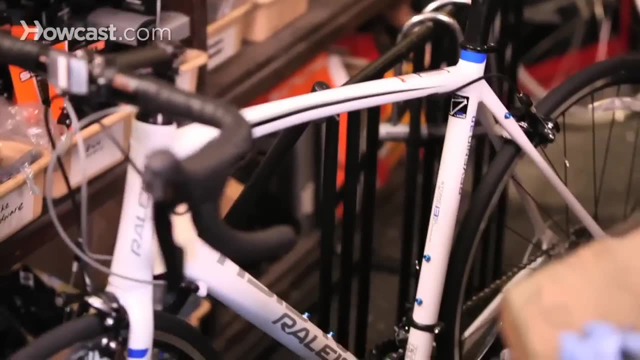 to put like a crowbar in there or like a car jack, something like that, and break them open. So let me demonstrate how that works real quick on this bicycle. Legally, you're not supposed to be locking to signs or street posts and things like that. 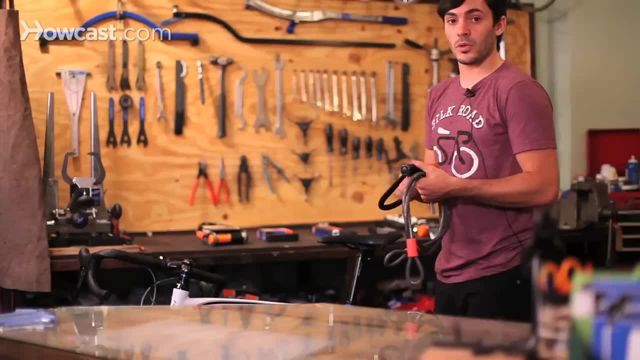 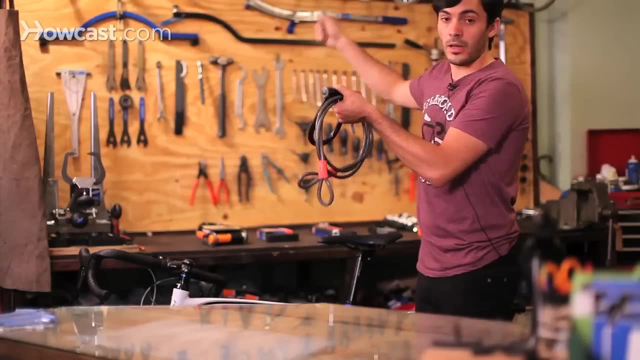 but a lot of times you don't have any other option. So just make sure that the sign or post has something at the top of it so somebody can't lift your lock up and over And take it right off. Also, never lock to scaffolding. 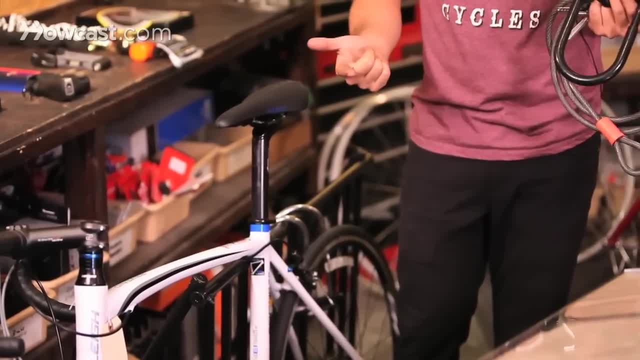 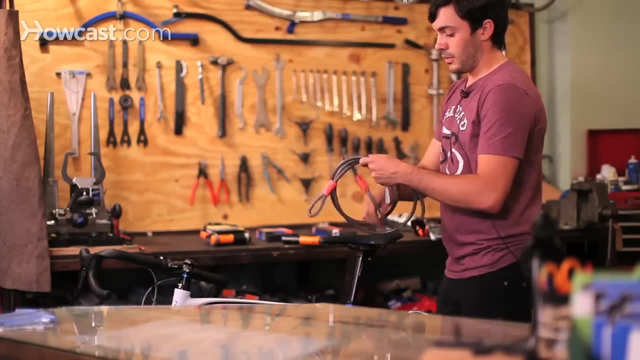 Scaffolding can be undone. Never lock to trees because it hurts the trees, and also the trees can be cut if they're small enough. So, basically, what you want to do is you go up to the rack and you're going to take your cable, unwind the cable and you're going to put it through your front wheel and weave. 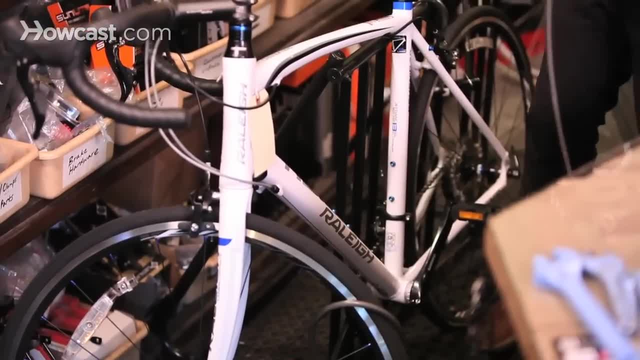 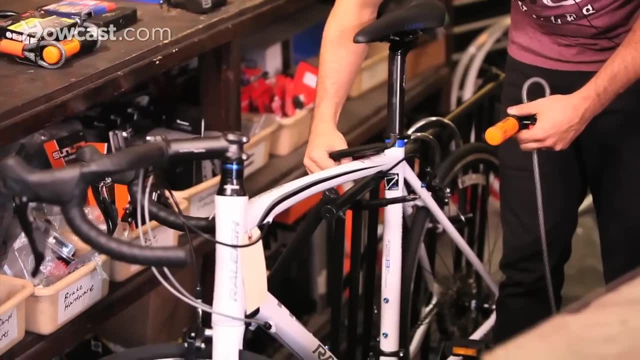 it through the hole here And then you're going to take your U-lock and you want to make sure that you're locking through the frame, Or if you want to protect your back wheel, a nice thing to do is to go inside this triangle. 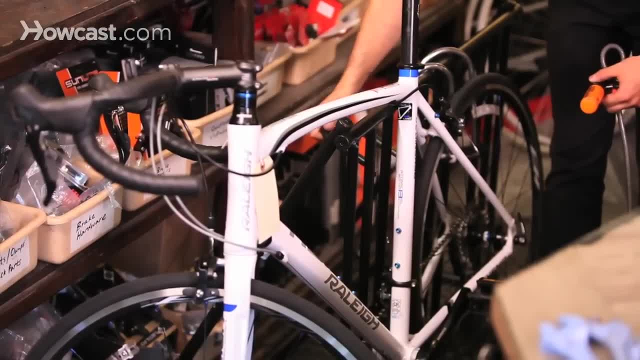 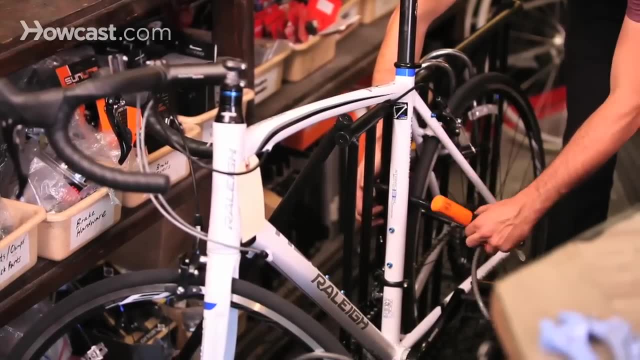 So you have a back triangle on your bicycle And you can actually go through. make sure you're attaching to the actual rack and go through and attach to the wheel, attach to the actual rim And then put the cable on, Make sure it's locked. 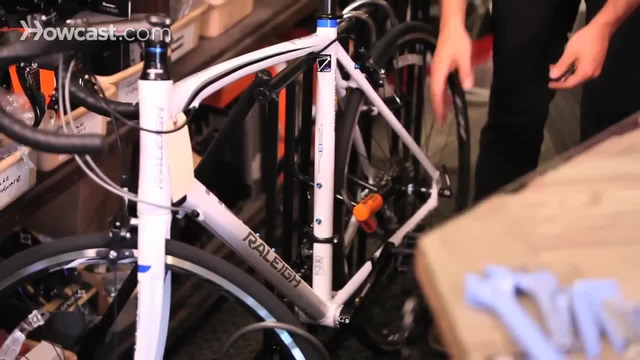 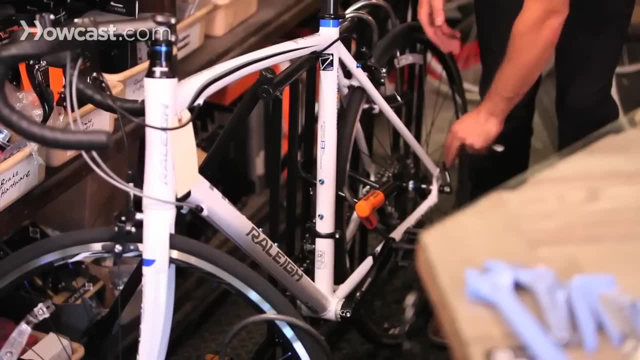 Give it a nice tug, Make sure it's locked securely. Basically, what that does is it locks your back wheel with the U-lock and your frame, Because even if you took the wheel off, it can't get outside the frame just because you're. 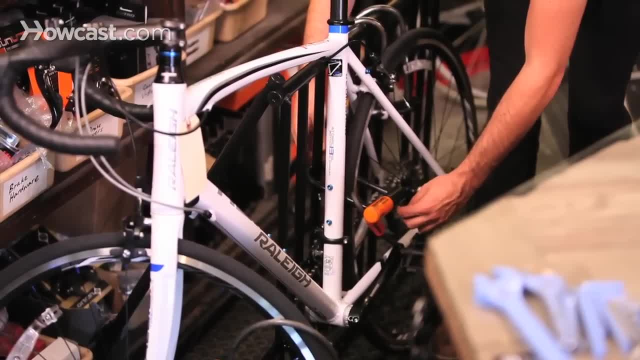 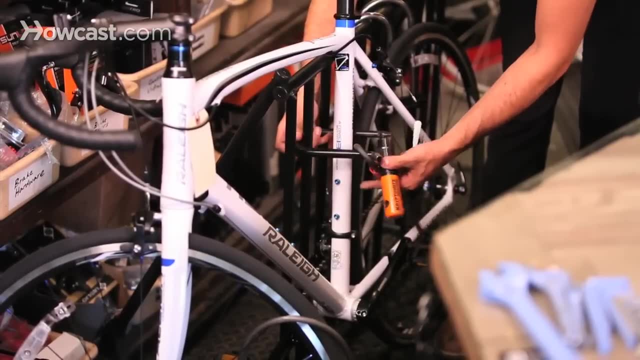 inside a triangle. So that's a nice way to lock it up. Or you can just if you're going into a store really quickly, you can lock up just to the frame and hope that your wheel is still there when you come back. 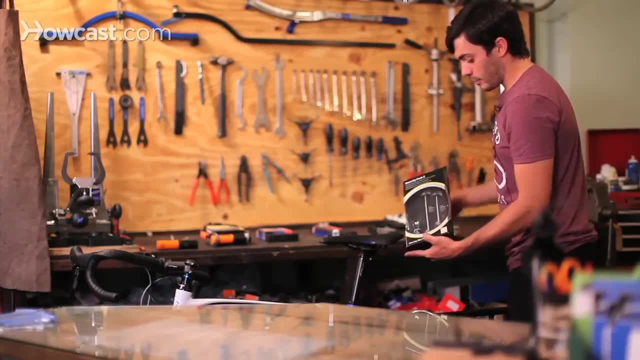 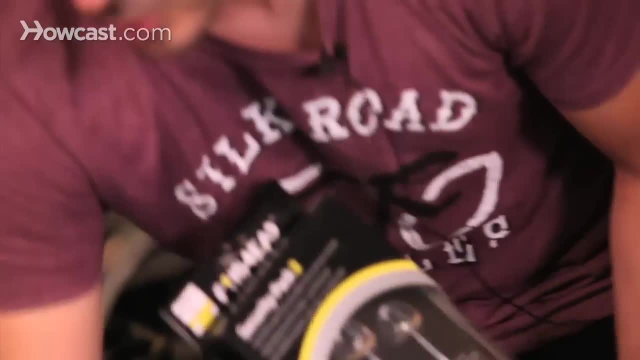 We recommend a lot of people get these pinhead locks. Basically, what it is is: it replaces the quick release and uses a key mechanism to keep them safe. It's a nice little thing because then you don't have to use this cable, You can just have the pinheads on. make sure you keep the key with you in your repair kit.